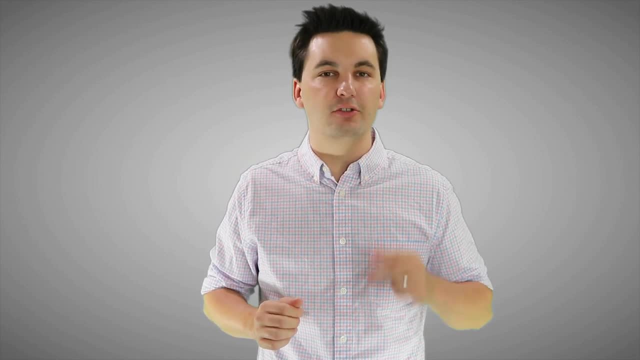 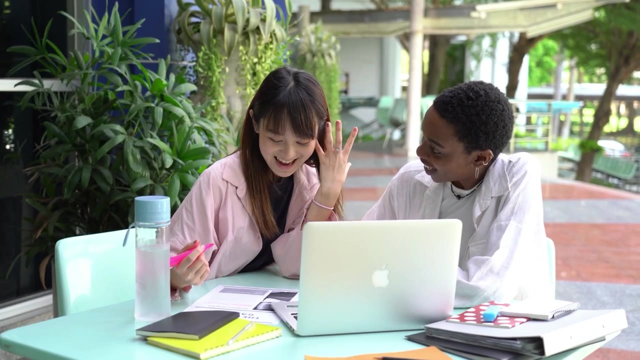 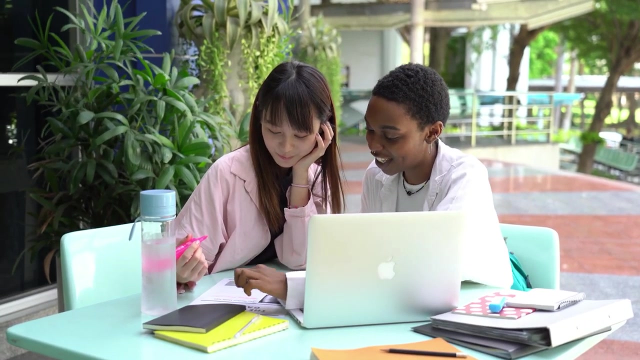 We're going to be looking throughout this video at different political, economic and social factors that are changing in society. Women are now able to get access to education and open doors that were never opened before. Not only are they learning new skills in school, but they're also learning how to be better mothers. 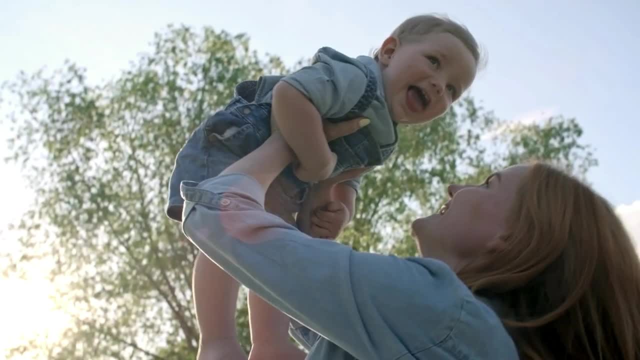 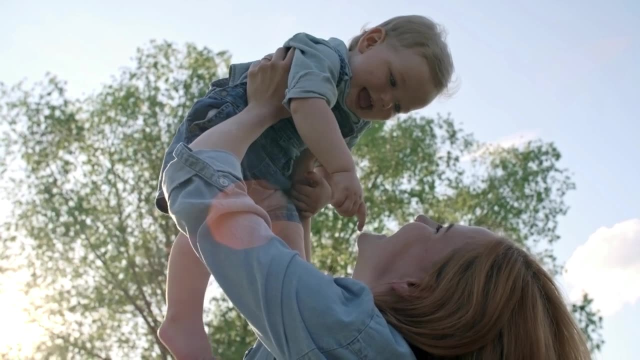 This is lowering the IMR, And when women feel confident that their children will live past infancy well, they're going to stop having as many kids. All of this decreases the TFR of a country, And as women continue to get education, they're more likely to then get higher education. 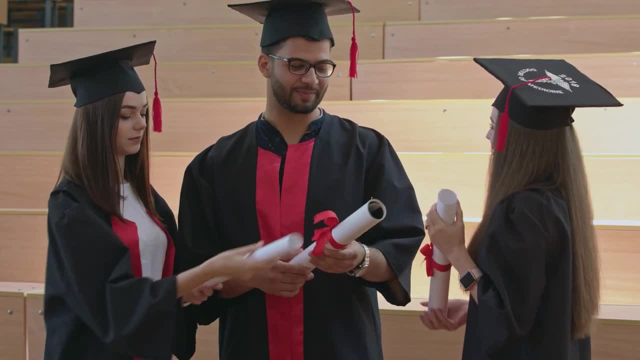 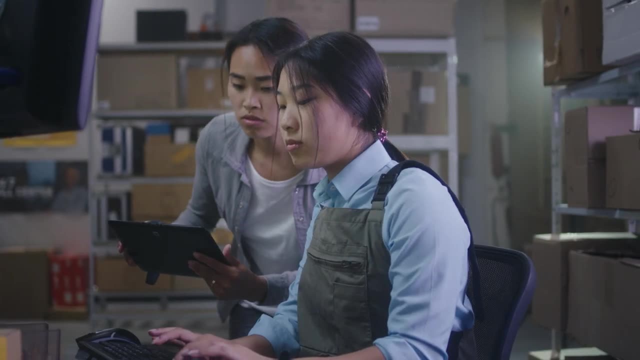 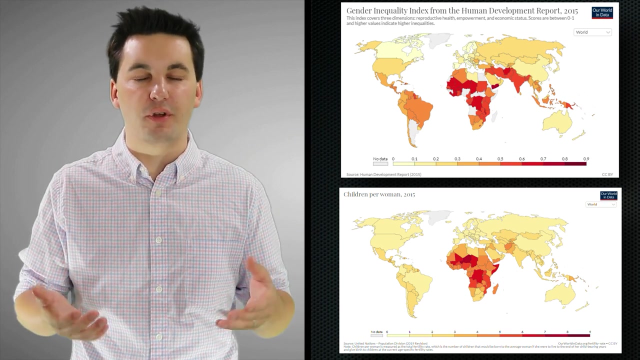 use those new skills. We are seeing trade sales in the workforce, Pursue careers, And all of this opens more doors for opportunities for women to be financially independent And it also reduces the amount of time they have to have children. When looking at the world today, we can see that countries that actually allow women to get educated 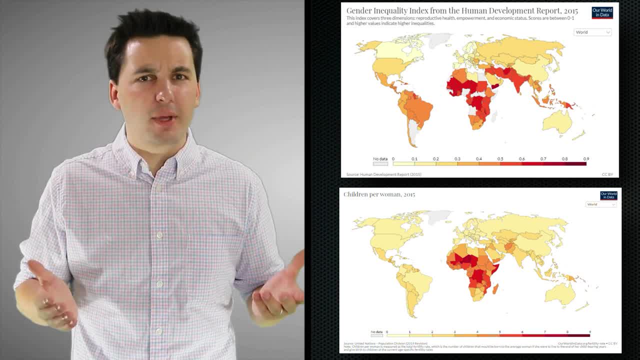 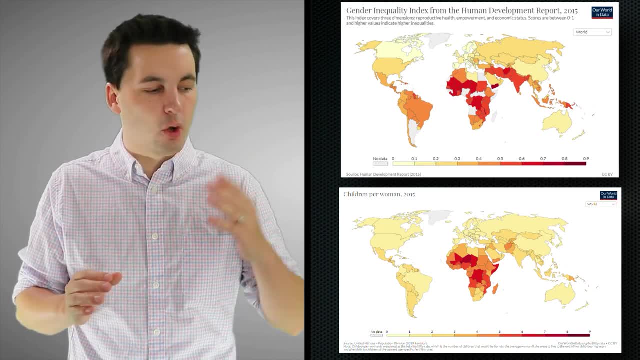 and also offer women economic opportunities, have a lower TFR. That's because women here don't have to rely on a man to be able to support themselves. Women can be financially independent. This allows them to pursue their own careers, their own goals. 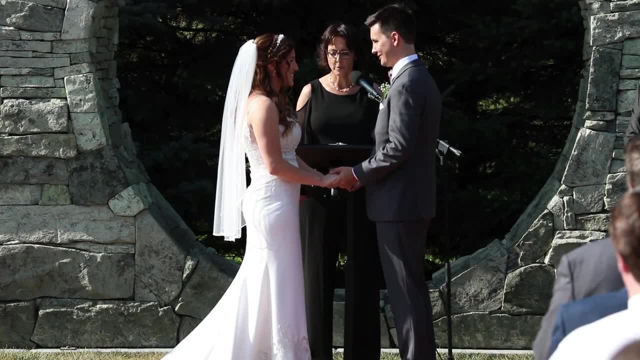 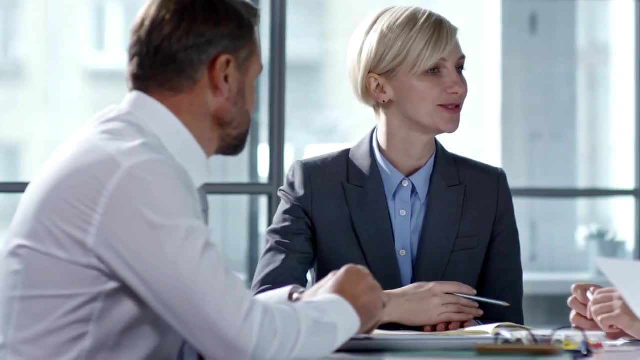 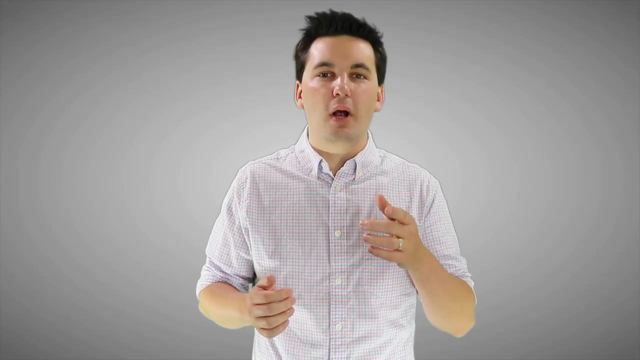 in society. This also pushes back the average time that people get married and also reduces the amount of time that people have to have kids. If women are now active in the workforce, if women are now pursuing other goals, they have less time to have large families, and all of this reduces a country's TFR, Since we're 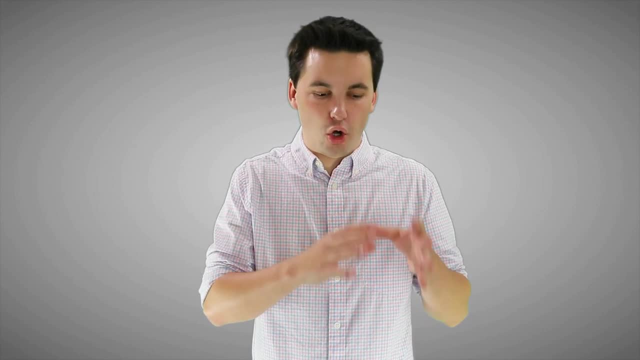 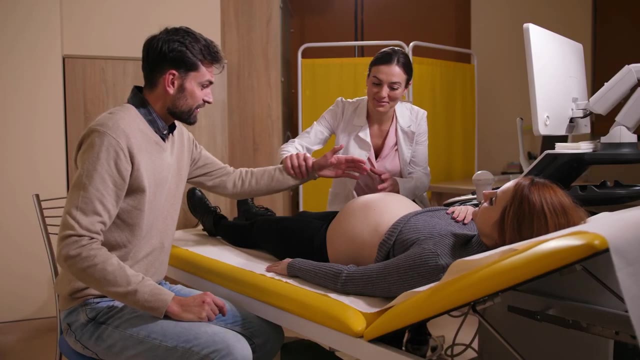 on the topic of economics, we could actually look at how the developed world is more urbanized and very career focused. If women have large families, they're going to have to take off for maternity leave frequently. This doesn't allow them then to get ahead in their profession, to be able to move up in the 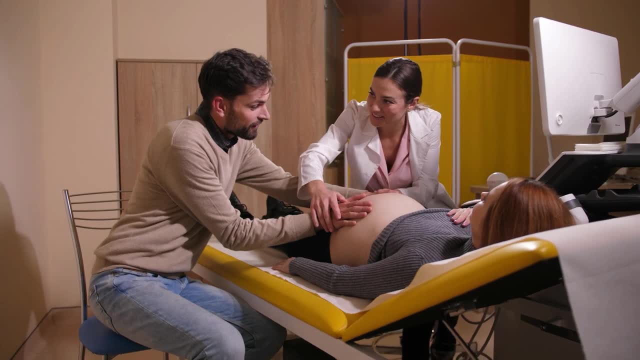 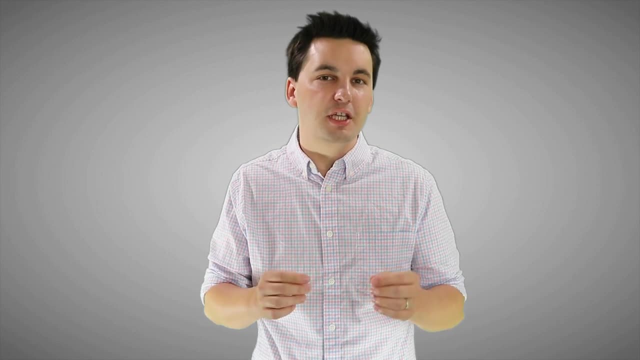 company. As they keep taking time off, they're not able to get as much done at work. Now, on the other hand, the developing world. they also still have to take time off after having children. However, kids in the developing world, particularly societies that are very agricultural focused, are seen as 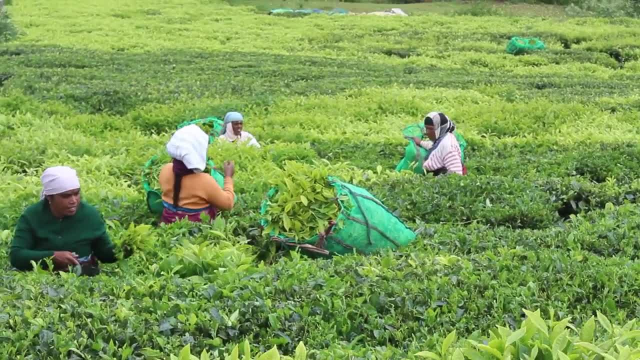 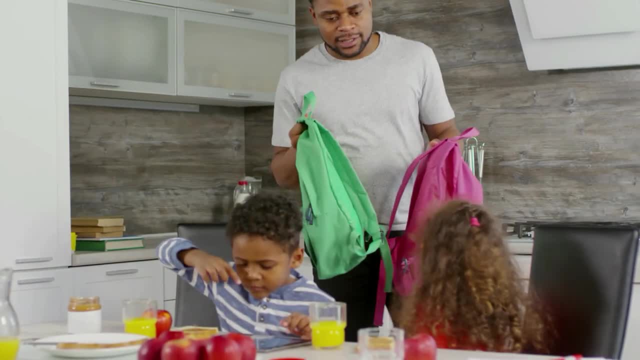 economic assets. They can help the women around the house with chores and also be able to help out on the farm with getting food and supporting the family, While in the developed world, again, kids aren't necessarily economic assets. They actually have a lot of money and they're able to make a lot of money and they're actually cost you a lot of money. Another factor that impacts a country's TFR is access to health care. access to medicine, advancements in health care- All of this helps lower a country's IMR. It allows children to live longer, which reduces family sizes. We also see that access to more doctors and nurses and 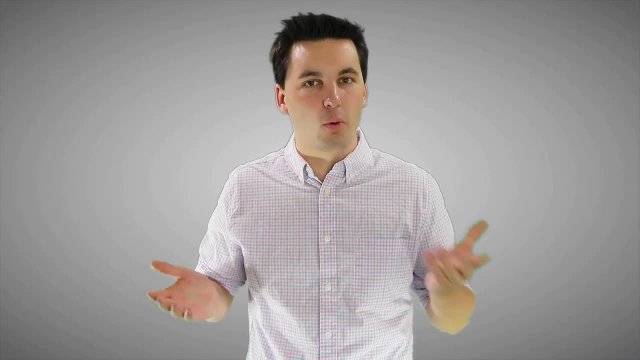 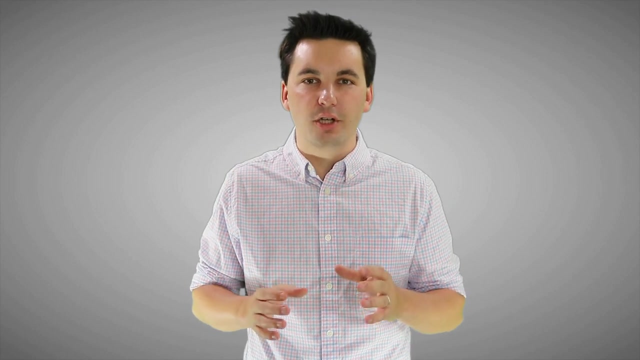 better technology will allow the mortality rate for women giving birth to also decrease. This is known as the maternal mortality rate, and really what's looking at is how many women unfortunately die while giving birth. the lower this number means. well, that means that society is more advanced. They. 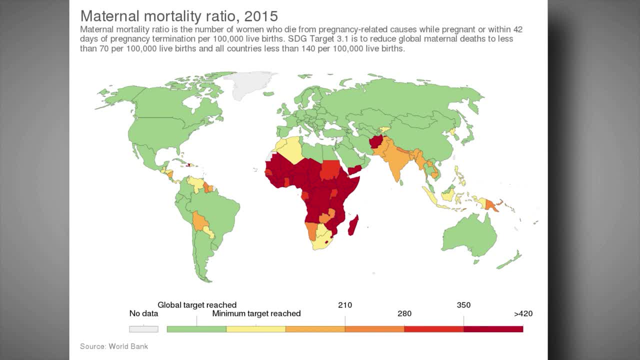 have better doctors and nurses and better resources to be able to help women be able to give birth. If that number is higher, that means that they're lacking these important services and unfortunately, that means that women aren't living through pregnancy. Now one last health care component we could talk. 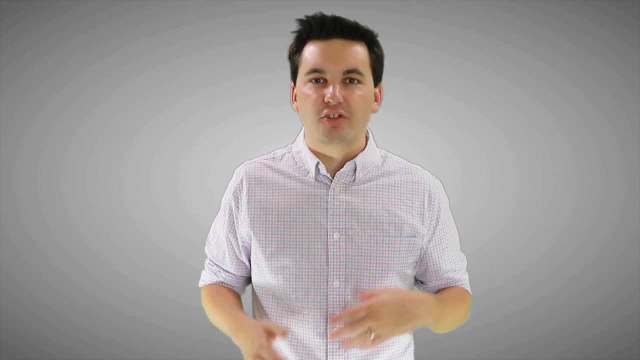 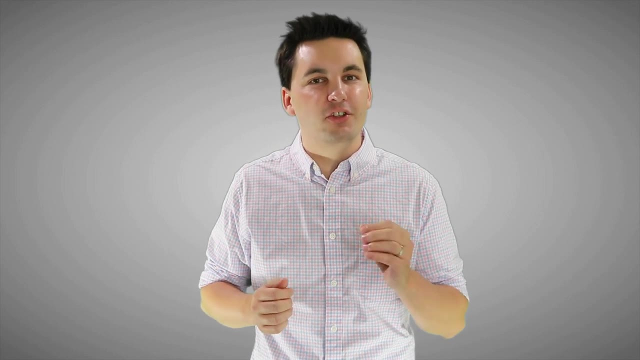 about. that's a little bit controversial is access to contraceptives. Societies that allow men and women to gain access to birth control or condoms will see that their birth rates actually go down. It's easier for families to use family planning to limit their family size, and all of this. 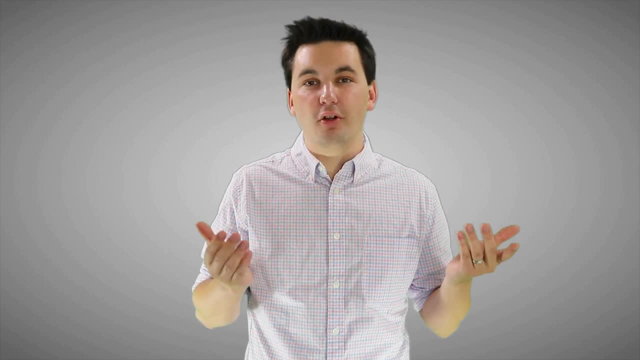 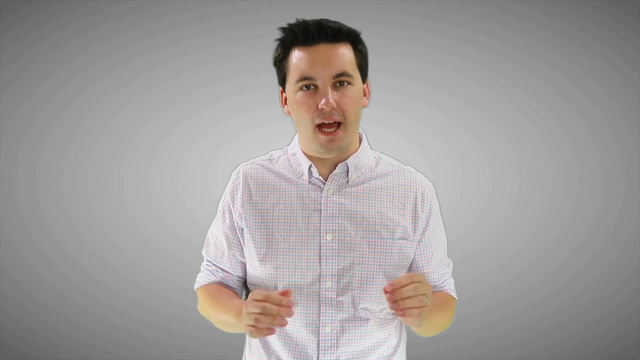 impacts on the country's TFR. Finally, we could also talk about political factors that will influence the country's TFR. Here we have our pro-natalist and anti-natalist policies and we cover these in depth in 2.7. so if you need, 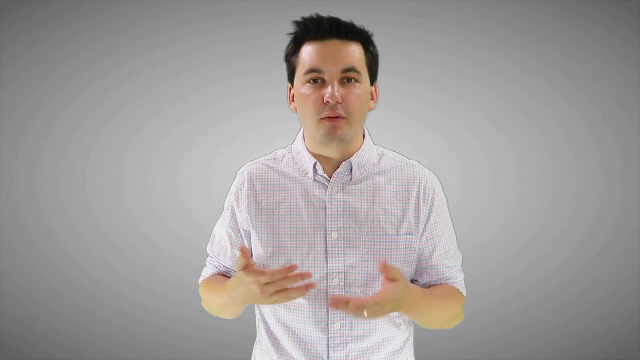 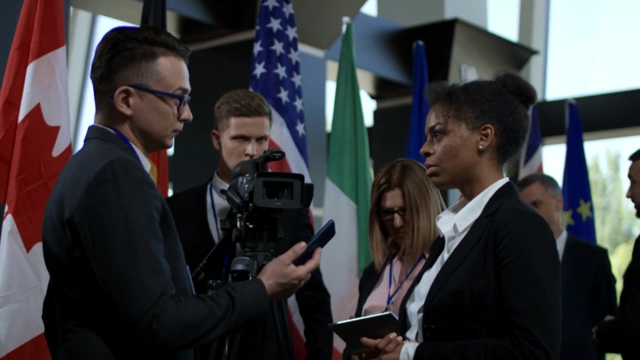 more information, go back and re-watch that video. But these policies have a big impact on if a country's TFR is going to go up or not, depending on how the government is going to allow women to have access to contraceptives or how they're going to reduce taxes for them. 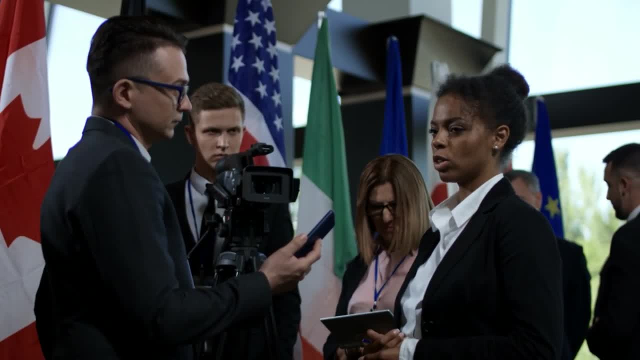 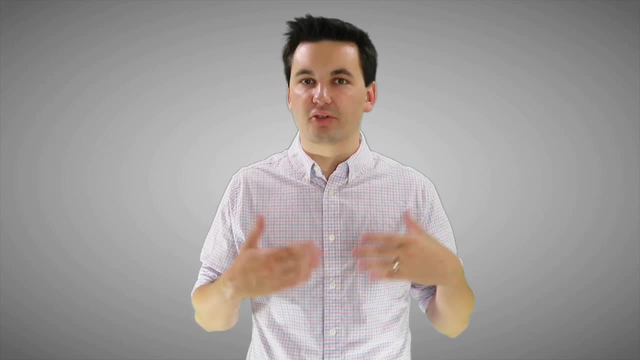 So we're going to be talking about these different policies that can impact people's behaviors and change the average family size for a society. Alright, now that we've kind of talked about different political, economic, some cultural factors that are changing in society, that have impacts women's roles. 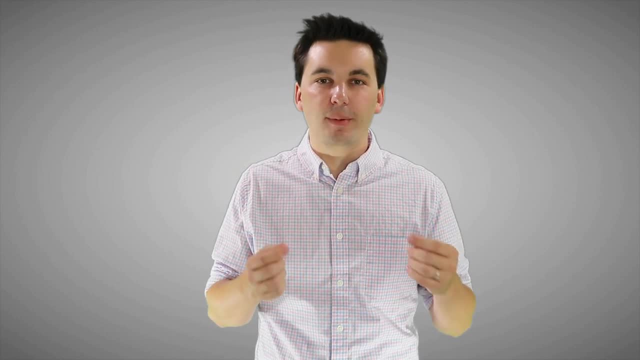 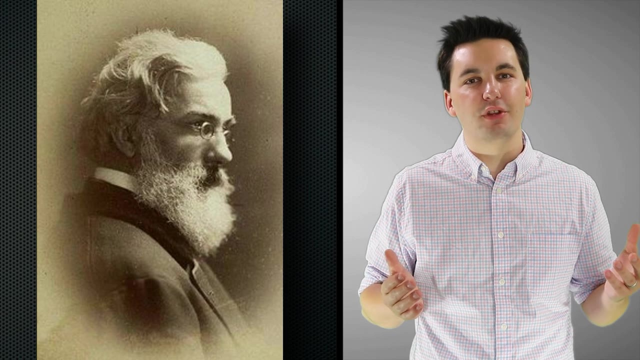 and also a country's TFR. we're gonna shift gears a little bit and talk about how these factors have actually changed migration patterns, and we're gonna be looking now at Ravinstein's laws of migration. Now Ravinstein came up with these laws to look at how demographic patterns and migration are happening in. 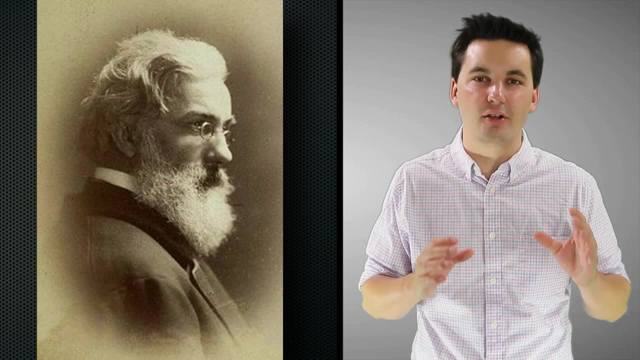 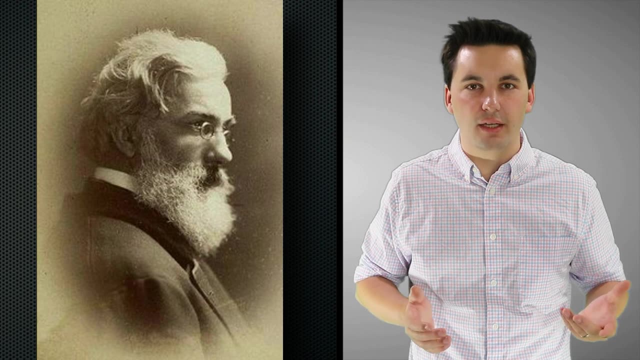 the world today and we're going to see that these laws are shifting a little bit, and that's because of societal changes: how we now view women and men in the workforce and in society. All of this has had an impact on the real world today, so don't worry about memorizing the order of these laws- in fact, I'm not. 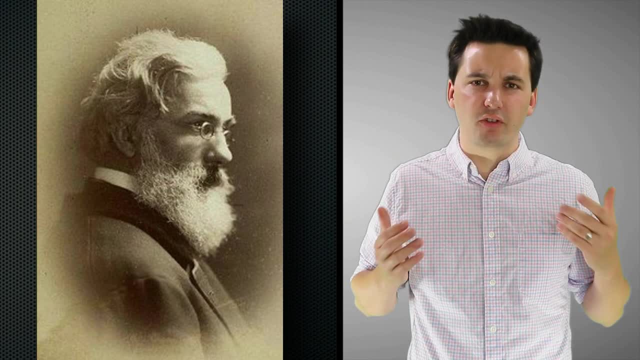 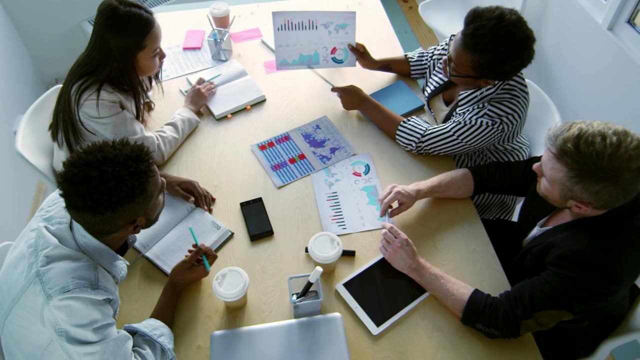 even really reading it in any particular order. instead, focus on the main concepts and focus on these themes and how they connect to our world today. One of the first things Ravinstein noticed is that most migration happens because of economic reasons and most of the people migrating are young adults. We don't see. 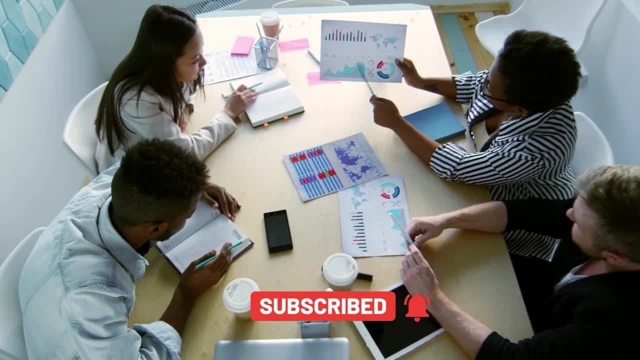 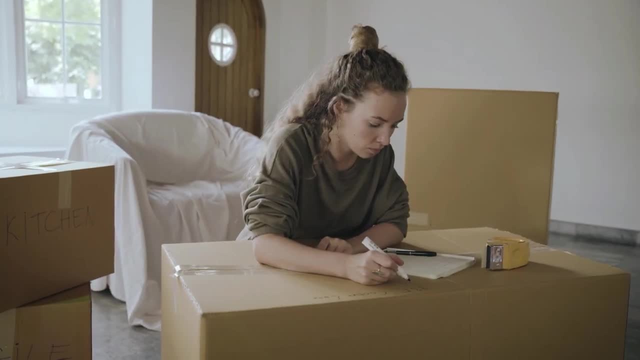 them migrating as much, particularly over international borders, and that's because it's dangerous, it's risky. Young adults have less things tying them down to one geographic area, and so it's easier for them to get up and move their lives. As you get older, it becomes more difficult as you start to gain more. 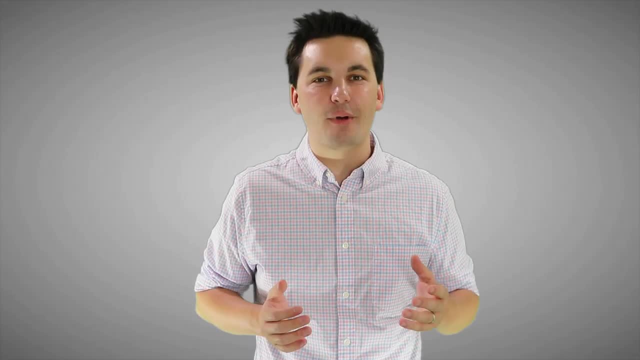 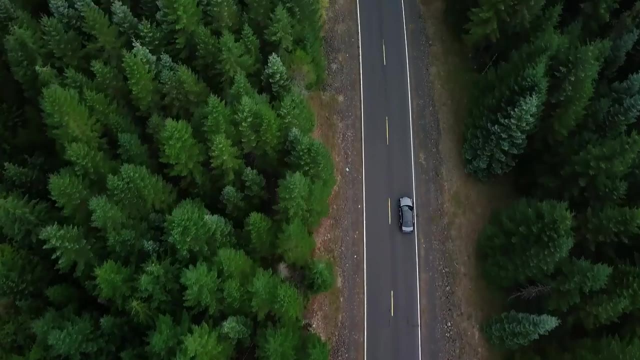 connections to the geographic location that you're living in Now. the next thing that Ravinstein noticed is that migrants actually travel short distances and they travel in step migration, and this makes sense. if I want to get from point A to point E, there's going to be some areas in the middle. I'm going to stop at a city. 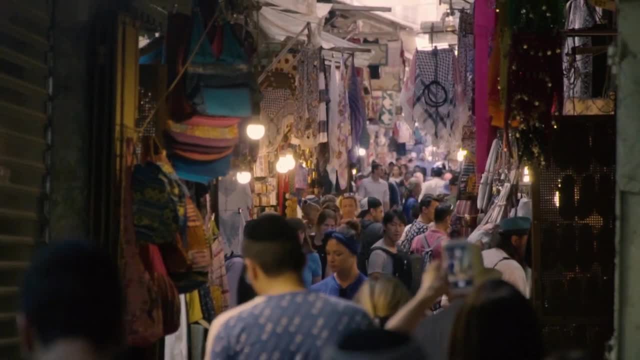 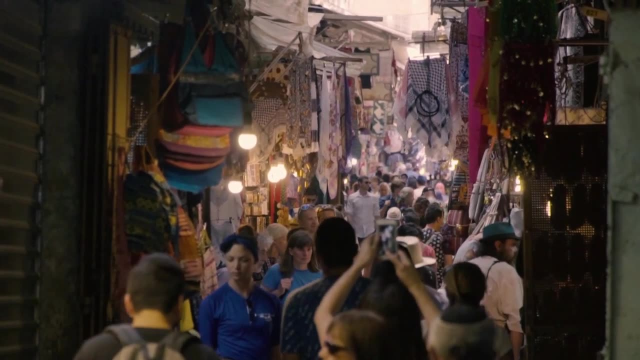 I'm going to stop at a town And I'm going to interact with places that are closer to me. Remember, this actually connects back to a concept we learned about in unit one, topic four: distance decay. We're more likely to interact with things right near us. 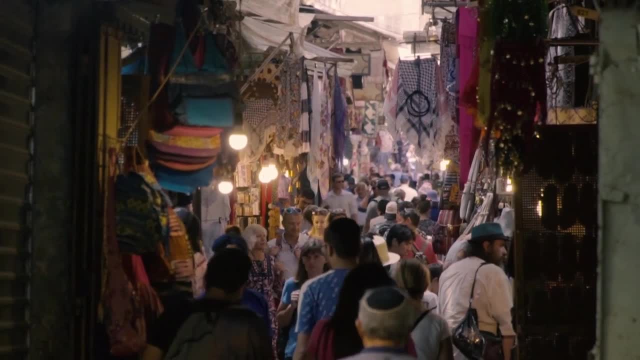 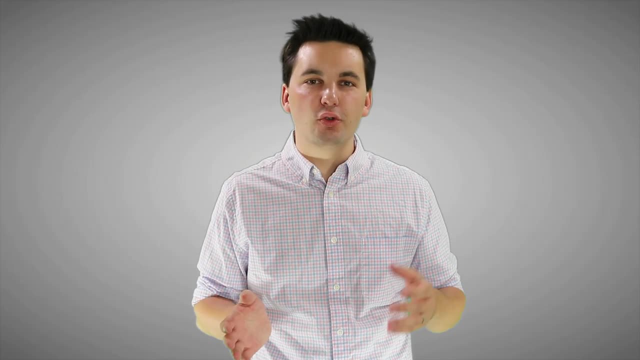 instead of things that are farther away. Now, over time, we've actually seen that, due to time-space compression and advancements in technology, people can now travel farther than ever before. And as Ravinstein continued to explore those first two laws, he then noticed too, that migrants are more likely to come from. 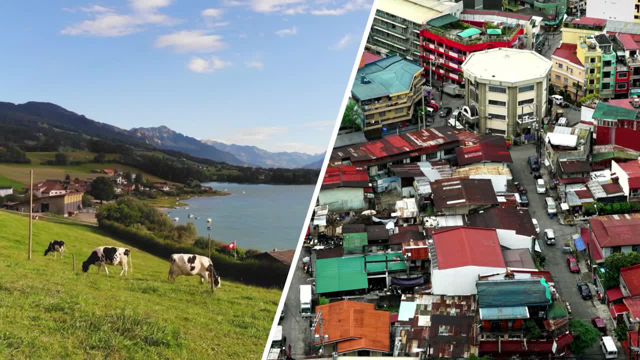 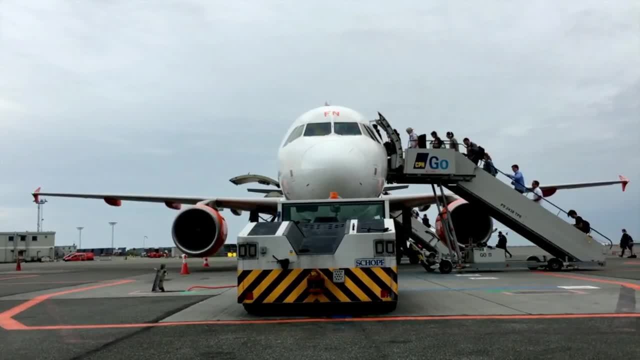 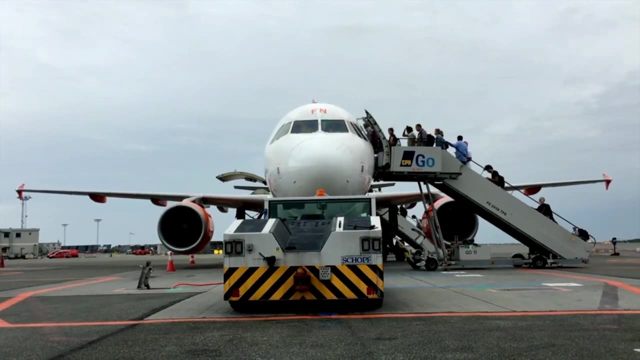 rural areas and go into urban areas. We're more likely to see people go from agricultural based society into a more industrialized urban area. That's because of the economic opportunities that they offer, and the farther they're traveling, the more likely it is that the migrants are going to be going to a very large urban area. And when migrants move, 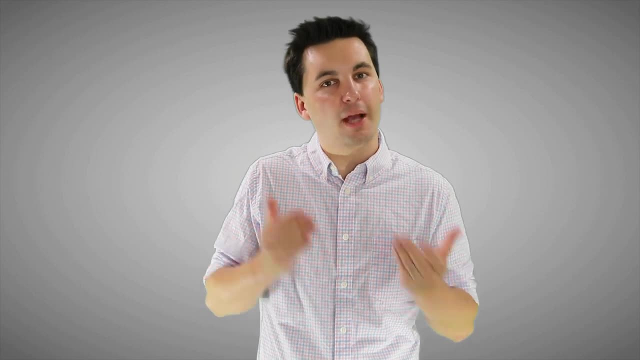 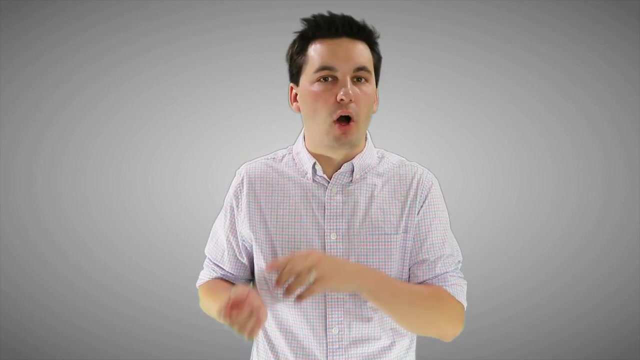 to a new geographic location. that now connects that new place back to their home and this creates a counter stream. An example this could be: let's say, college graduates from Florida move all the way up to Rochester, Minnesota to work at Mayo Clinic, and then people from Rochester Minnesota 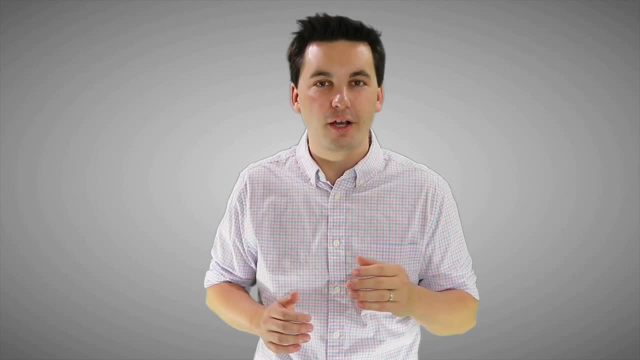 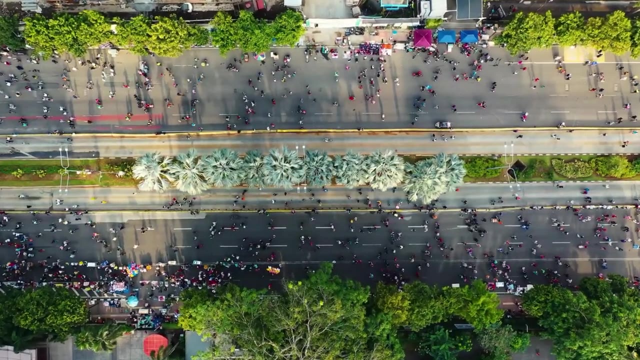 move down to Florida because they heard how great it is there to retire and enjoy that nice weather. These two locations are now connected. One thing to note about the counter stream is it doesn't mean that there's going to be the same volume between two different geographic locations. 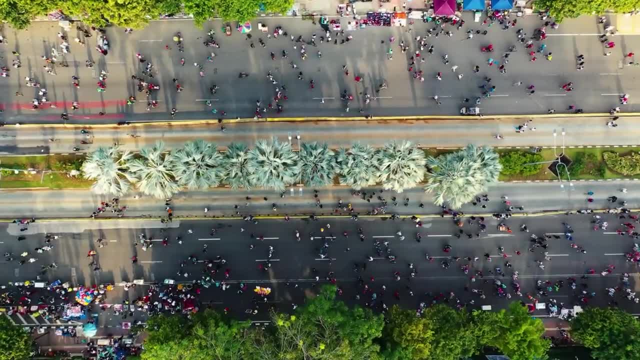 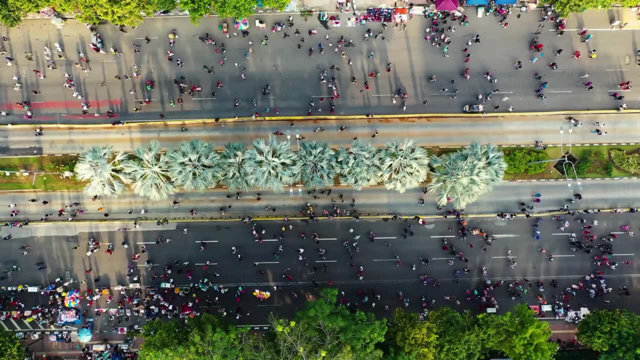 If migrants move from point A to point B, we're not going to see necessarily the same amount of migrants moving from point B to A. There is going to be interactions between these two places now, but it's not necessarily the exact same amount. The next thing that Ravinstein noticed was that 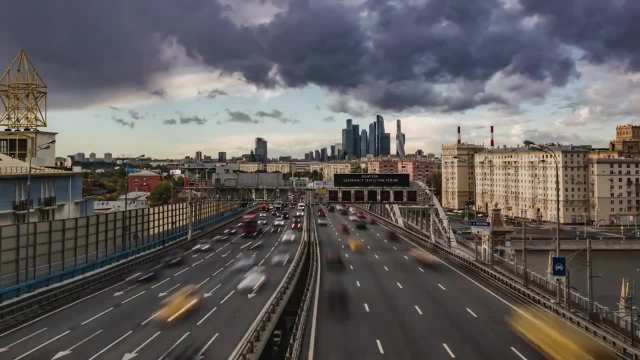 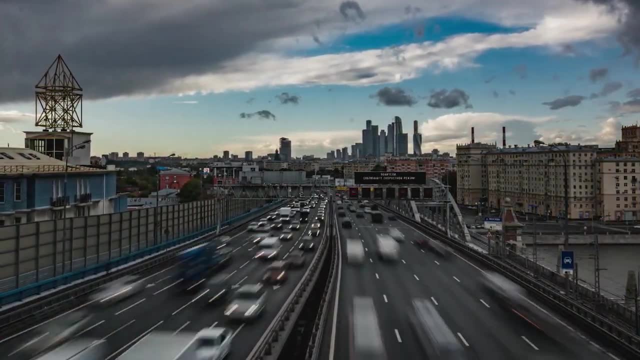 large urban areas actually grow through migration. They're not going to be growing as much through their natural bursts anymore. Their TFR is too low and that actually connects to the gravity model. Large urban areas have a lot of pull factors. They offer a lot of economic, political and social opportunities for citizens that smaller 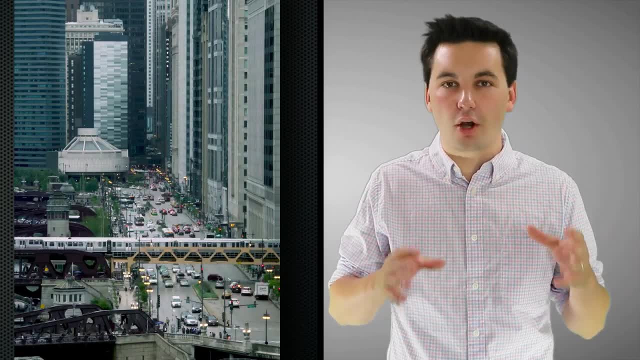 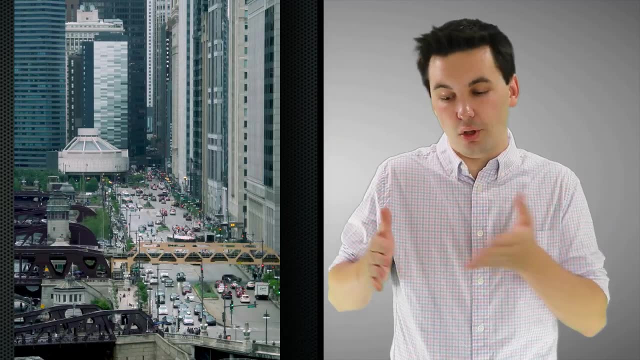 communities just simply don't have. And so we can actually see that large societies, large urban areas are going to attract people from farther away, compared to smaller settlements that might be closer to the migrants. They're going to go to the large areas because of all the economic 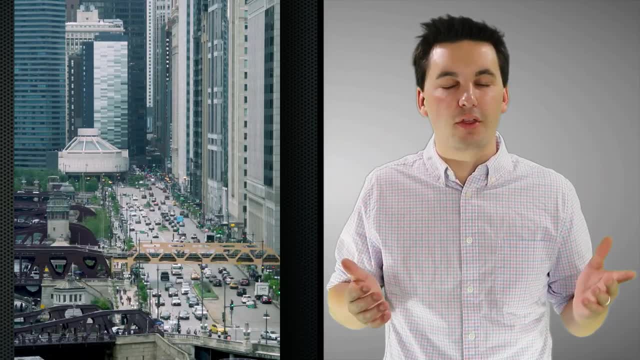 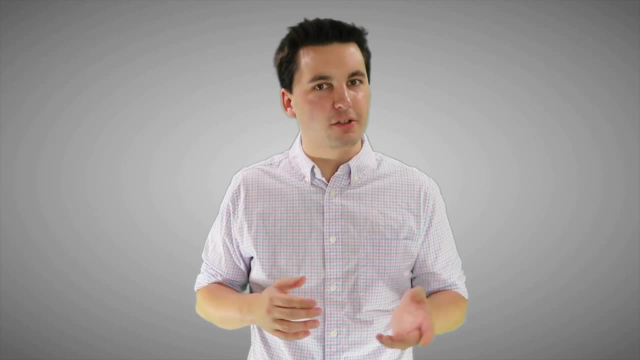 political and social social opportunities, And here we can also see, too another law that Ravenstein noticed is migration equals more economic development. Now, one of the last things that Ravenstein noticed was that women were more likely to internally migrate within a country's boundaries, while men were more. 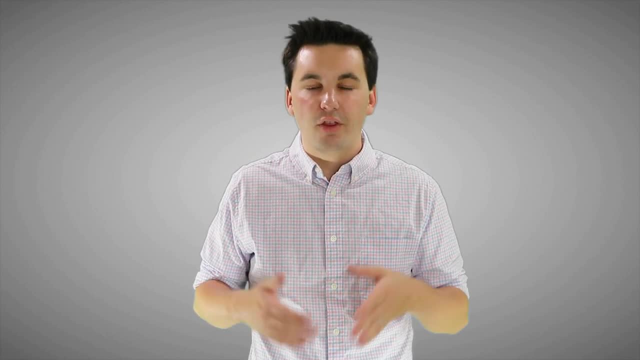 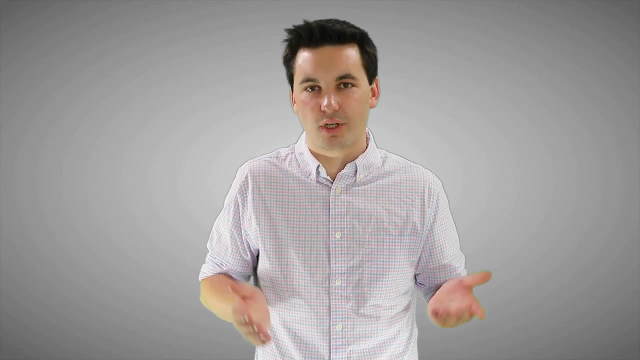 likely to cross an international boundary and migrate to a different country. This was because men were seen as the caregivers- the ones who are going to be the providers- and had the financial capability to be able to migrate to a different country. However, today we can actually see that 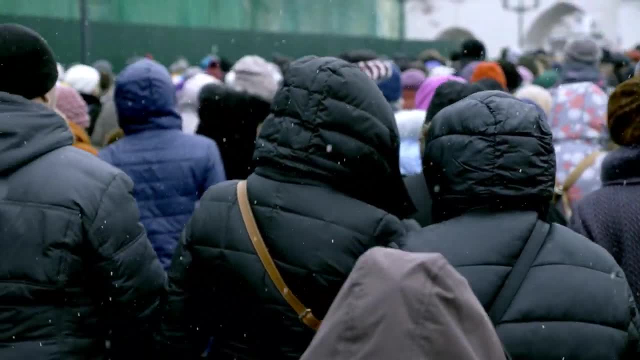 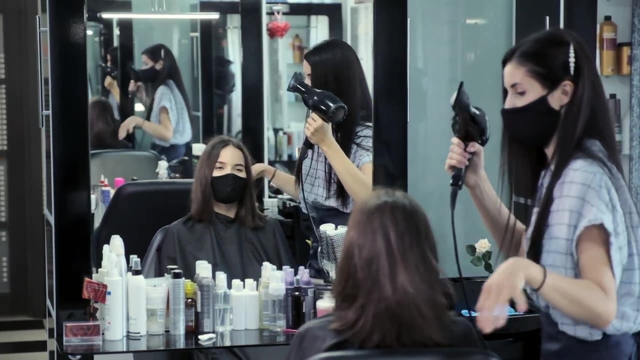 this law is kind of changing as more and more women are now crossing international boundaries. This is because women are able to actually work now and be providers for the family and have access to financial resources that allow them to be able to migrate to a different country And as 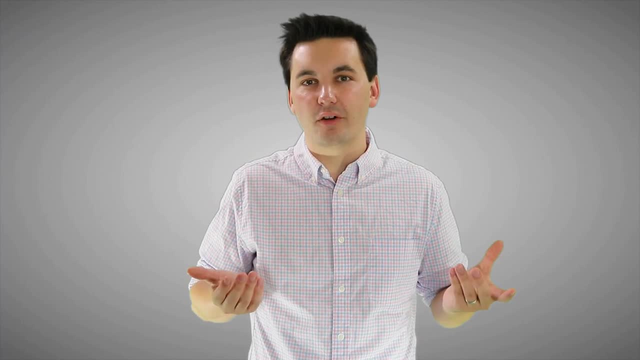 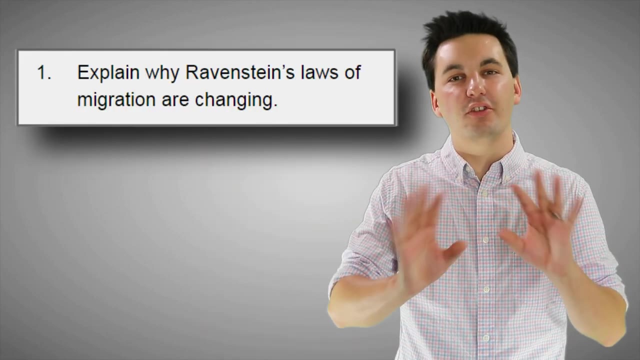 women continue to gain more rights and opportunities in society. it's only a matter of time until Ravenstein's laws continue to shift again And we'll have to wait to see what happens And just like that, we're done with 2.8.. Now, this isn't new to you. You know the drill. Answer the questions. 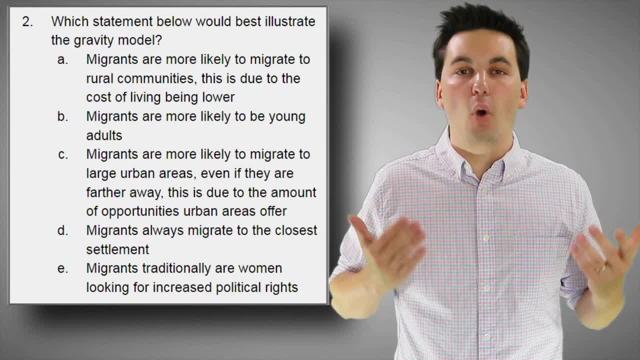 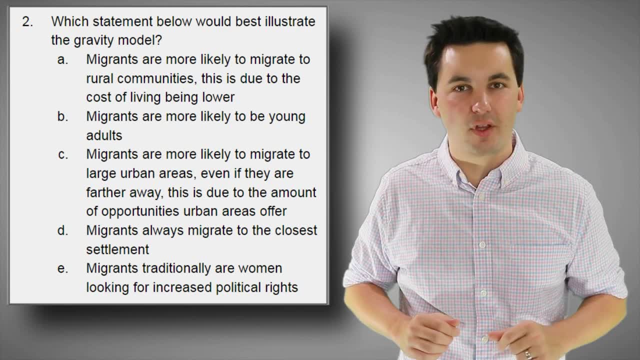 on the screen right now and then check your answers down below. And if you haven't already done so, please do so now. And if you are struggling with AP- Human Geography- and you need a little bit more help, don't forget to check out my Ultimate Review Packet. It'll help you get an A in your class and a 5 on that. 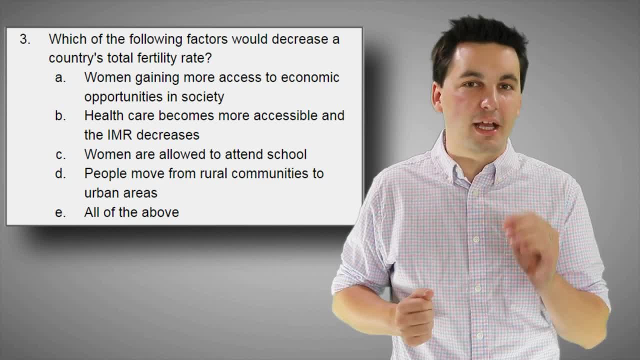 national exam. Alright, that's all the time we have for today. I'll see you next time when we talk about aging populations with 2.9.. I'm Mr Sin, and until next time, geographers. I'll see you. online. Thanks for watching.